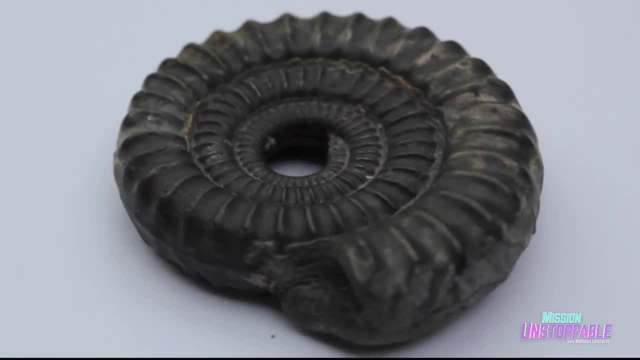 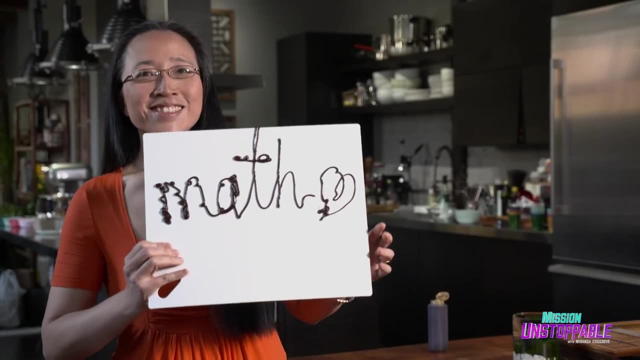 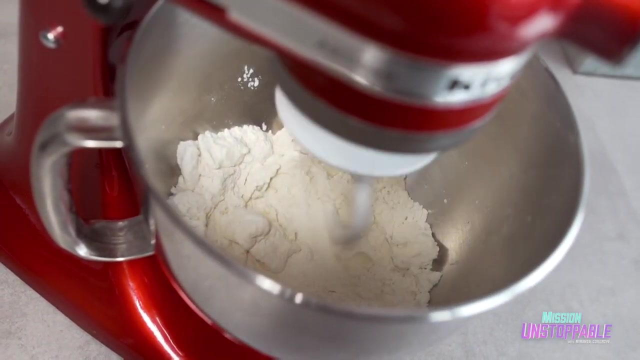 can be. Pure math is about studying one thing and seeing a pattern and then asking: well, if that's a pattern, then where else can I find that pattern? And today, mathematics professor Dr Eugenia Cheng is going to help me learn more about pure mathematics by baking. I really love. 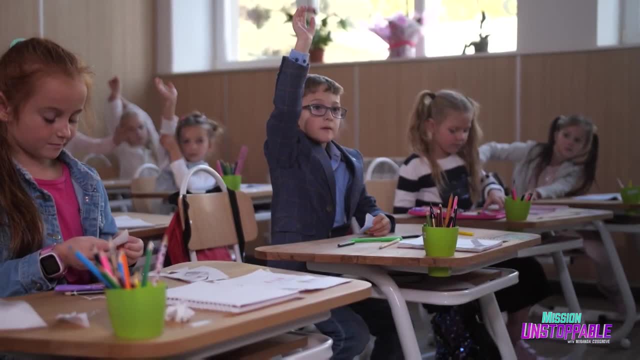 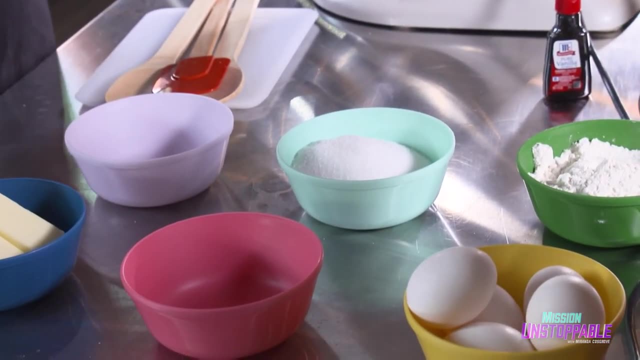 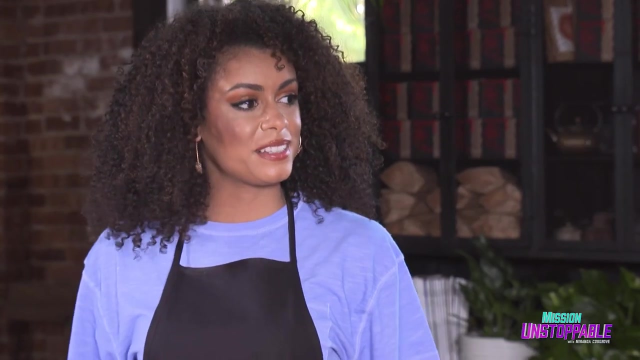 understanding how things work like when little children keep asking why, but why, but why. I was like that and I never stopped asking why. Welcome to the kitchen where baking and math join together to make delicious and logical math. I hear that you're a pure mathematician. What even is that? 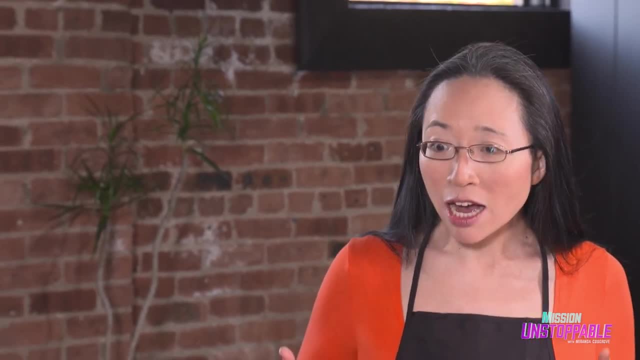 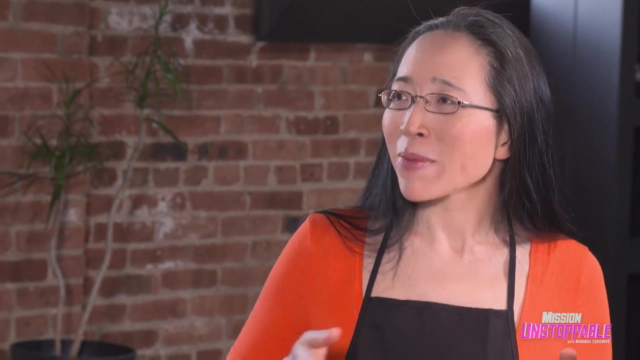 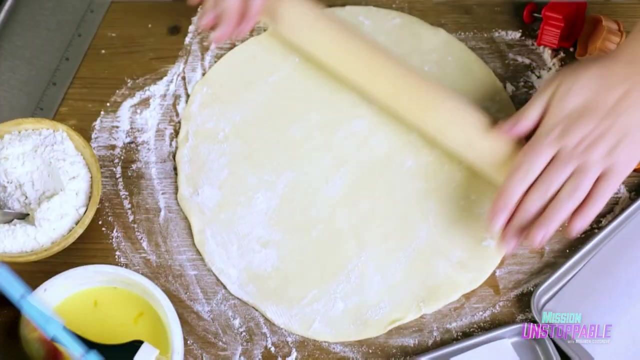 Pure math is about spotting patterns and understanding how things work, often so that you can make things yourself. Let's start with pie. What makes a pie a pie? I'd say it starts with a crust and then some fruit filling a second crust on top. 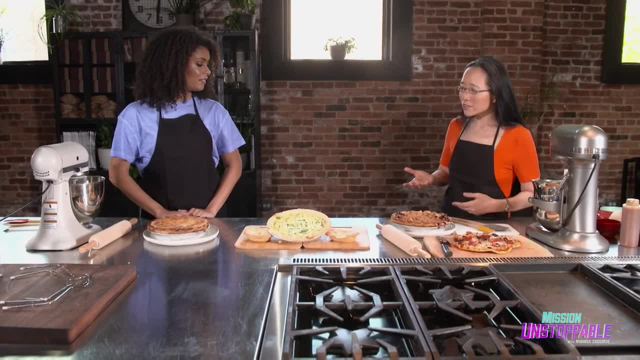 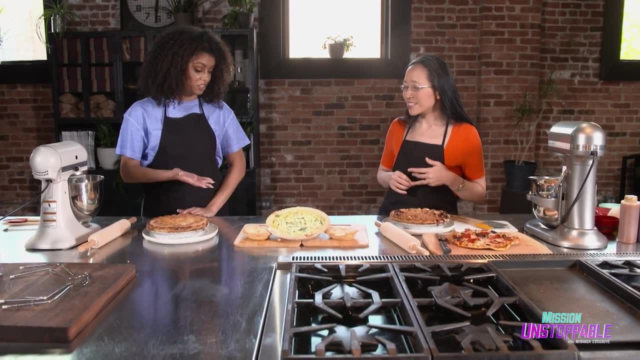 and then you bake it. But what about this? Is this a pie? It doesn't look like a pie. It doesn't seem to have fruit in it. No, it's a quiche, but I could see why I would call it a pie. 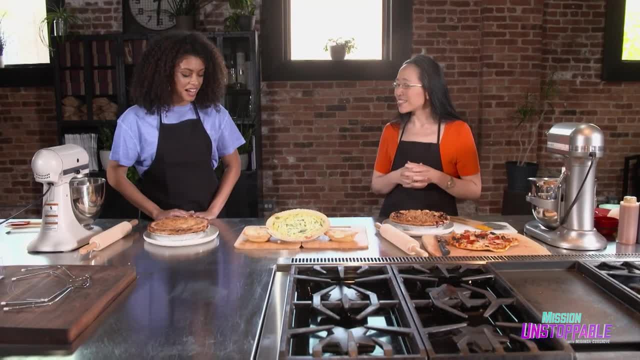 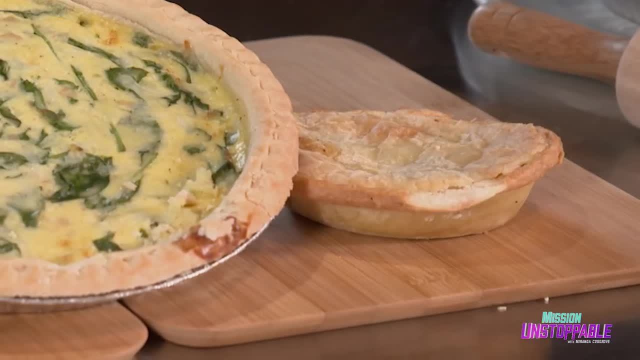 And what about this? Is this a pie? Actually, chicken pot pie is one of my favorite kinds of pies. Chicken is not a fruit, But it still could be classified as a pie. So if we define pie as something with at least one crust and a filling, 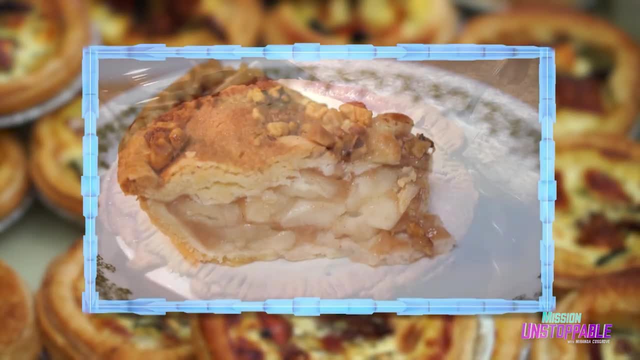 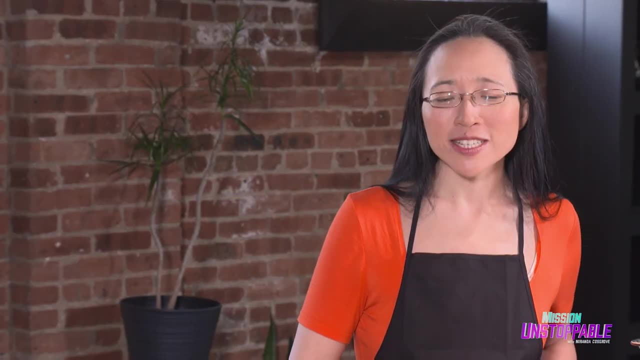 then we can make an endless number of pies: Apple pie, cherry pie, shepherd's pie, pizza pie. I guess math really is as easy as pie. Let's move on to cakes and we'll put abstraction to work. Have you heard of a Battenberg cake? 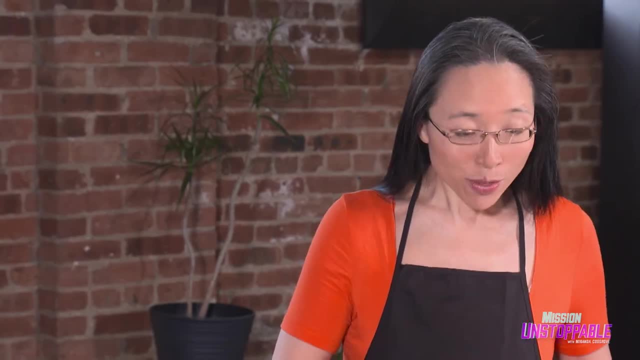 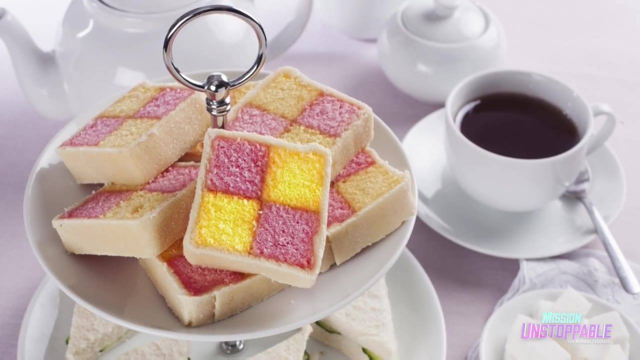 It's a great example of an abstract mathematical structure, So I thought we could make some- Ah, that sounds great. A Battenberg cake's distinctive two-by-two check pattern alternates pink and yellow. Wait, wait, wait, wait. I promise this will tie back into pure math at the end. 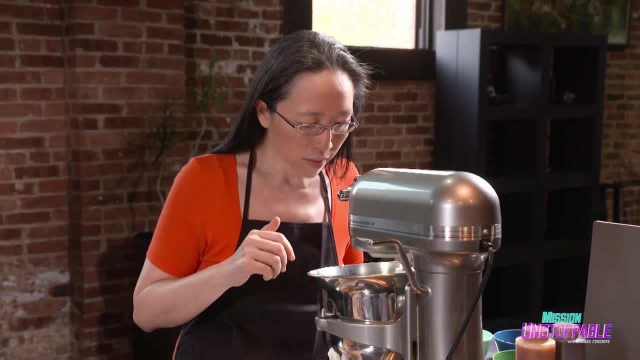 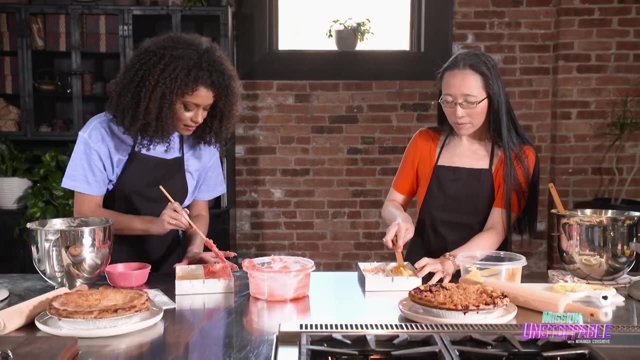 To make the cake batter we mix butter, eggs and sugar, eggs, sugar, flour and baking powder. Then we add pink food coloring to half of the batter. We pour the batter into a tin and add dividers to keep the colors separate. 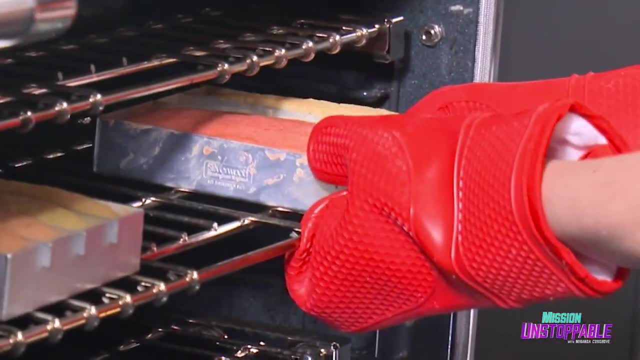 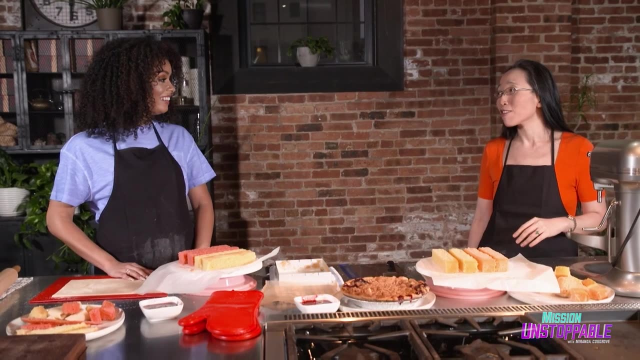 And after 30 minutes in the oven. So now the key is the Battenberg pattern. We have two colors of cake and we don't want the same color of cake to touch the same color of cake, because that would be terrible.